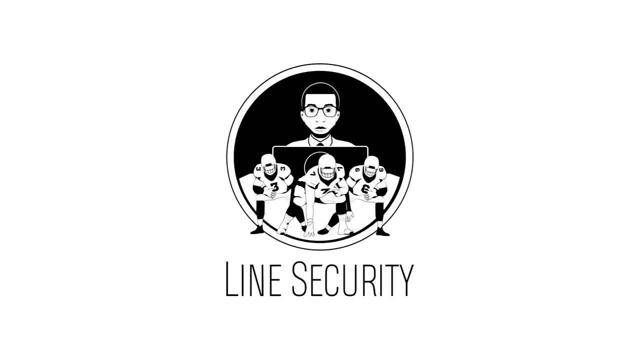 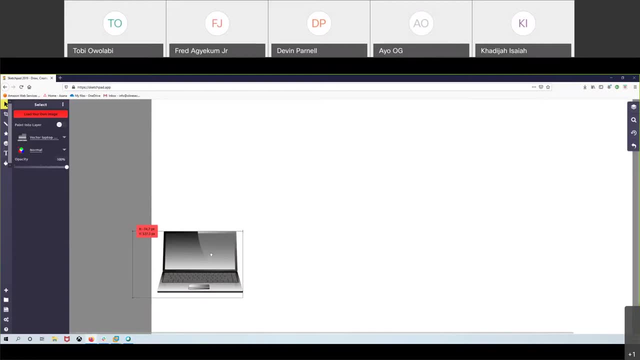 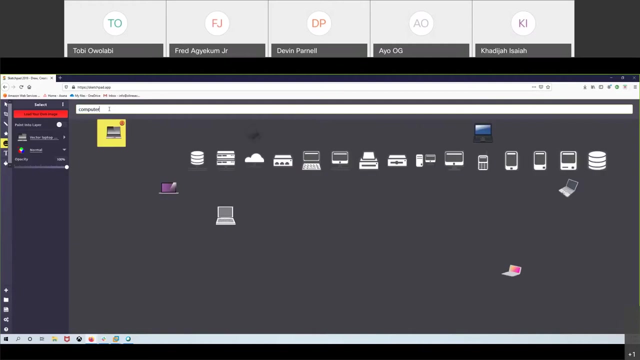 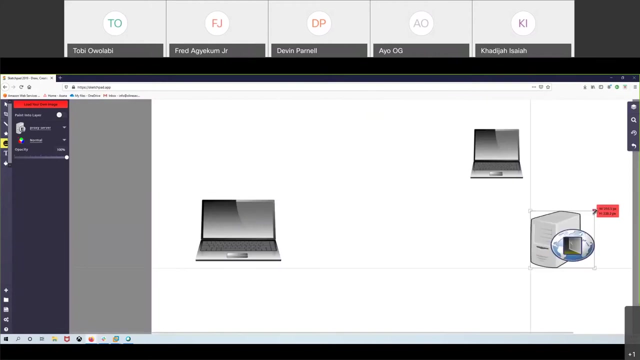 All right, so IPSec, like I was telling Ralph and Fred, it's really really simple. What complicates it is it being new information. That's really it, Computer. let's get a server. Let's get this web server. This is our web server over here. 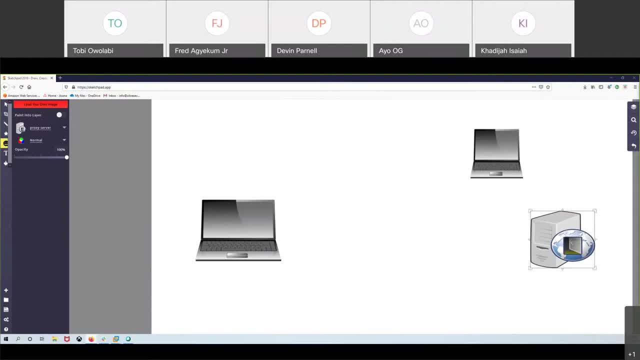 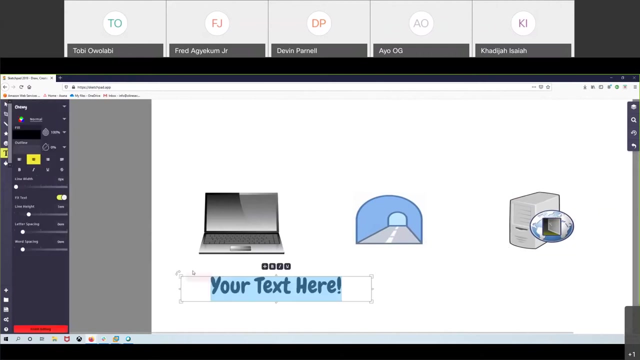 I need a tunnel. I like this, All right. Okay, so one more time. we're getting ready to just give you a different visualization of IPSec. All right, we're all set now. So we have you the end user. The end user is the person using the laptop. It could be a phone, It could be a. 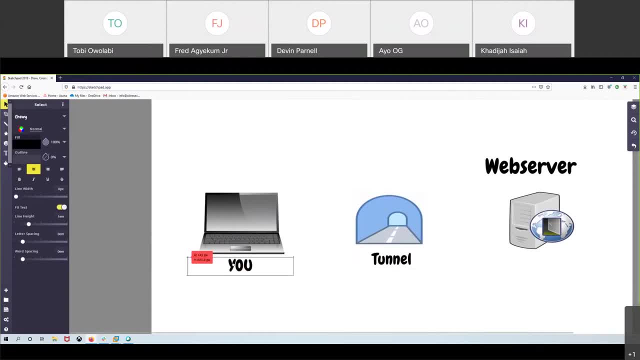 tablet, a workstation, whatever device you're using. For our scenario here, we have a laptop And you happen to be at home during COVID, But your company does not trust your home network. Your home network is your Wi-Fi, whatever you use to connect to the internet at home, That's. 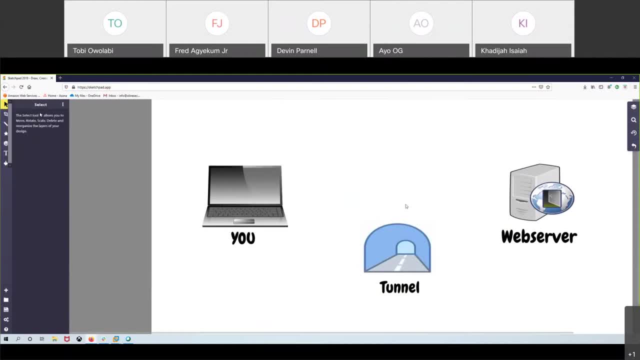 your access point, It's your router, It's your Wi-Fi. So, since your company can't trust your home network because they don't have control over it, they can't scan your home network as many times as they do the company's network. 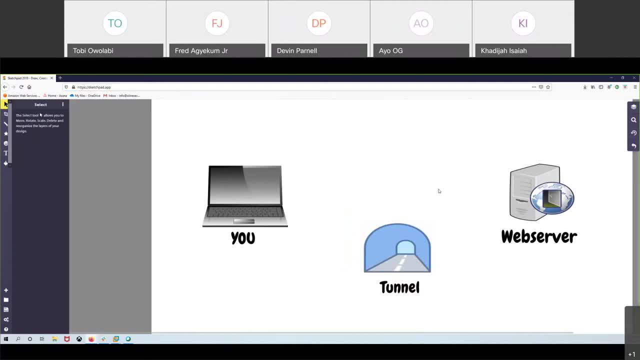 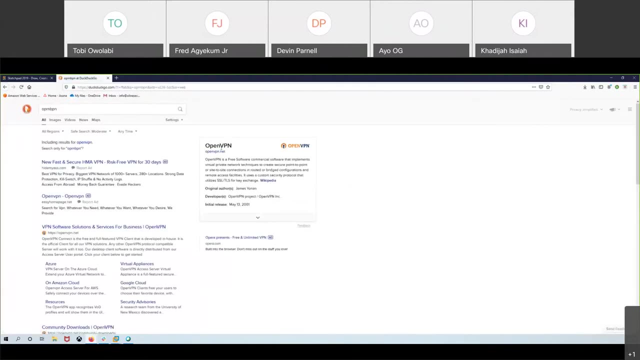 So they have. you install a VPN on your laptop. You can go and install a VPN anywhere you want to Open VPN. I put VPN, But you can install a VPN. They all work the same. There are different ones out there, They're all the same. 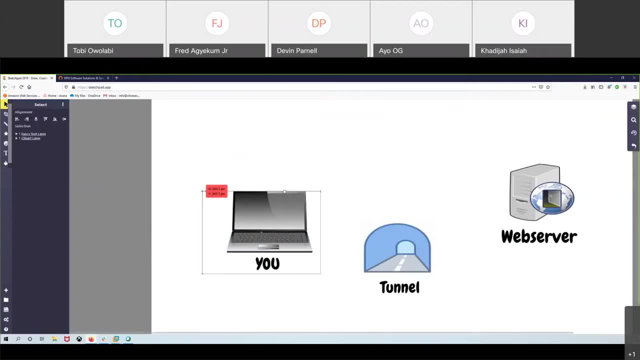 So they have you install this VPN on your laptop. Right here we have a VPN installed on it. We went to openvpncom and we installed it. Now you're using the VPN to connect back to this guy safely. Your company doesn't know if your network is safe. You could have an open network at home. 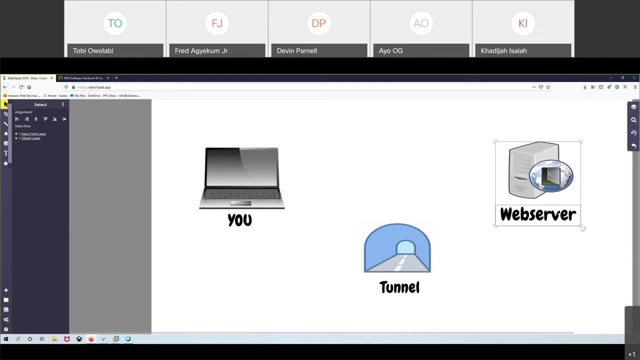 which means you don't use a password to connect to your Wi-Fi That's open, like airports, hotels, coffee shops, Open networks. They don't require a password. So you're using this VPN. Hey, quick one Yo. 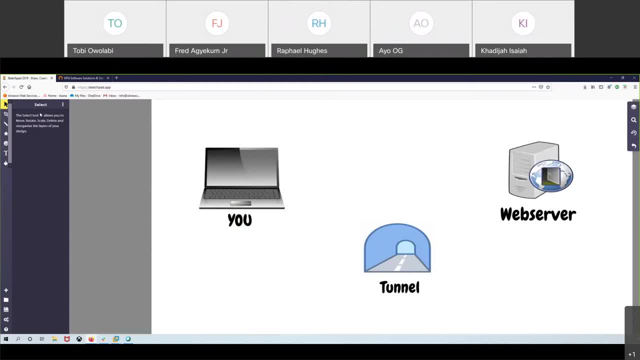 I was going to ask, like, if you use a VPN- I don't know, I didn't mean to take this off, but if you VPN in an airport, it would make your traffic safe, Exactly. So let's say we're in an airport right now You're trying to get to. 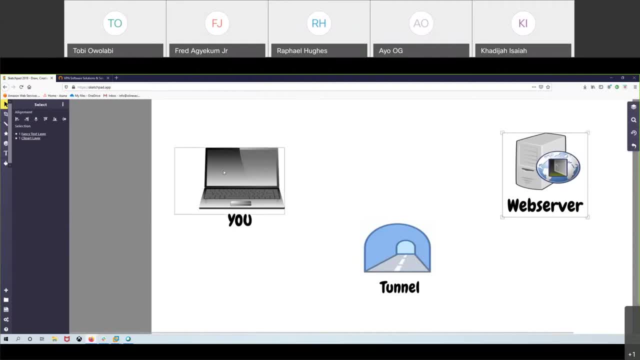 onlinesecuritycom right here on this website. You're trying to get to onlinesecuritycom right here on this web server. If you're not, if you don't have a VPN, I can see everything you're doing when you're on onlinesecuritycom. If online security isn't encrypted, it is encrypted. 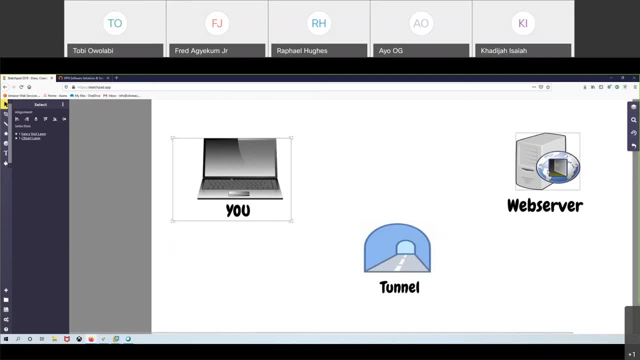 but let's imagine it wasn't. Let's imagine the website wasn't encrypted. It doesn't have that lock icon next to the web browser that Shondre showed you all. If it wasn't encrypted, everything you do on that airport's network, which is open, I can see it. Just like we said, we're. 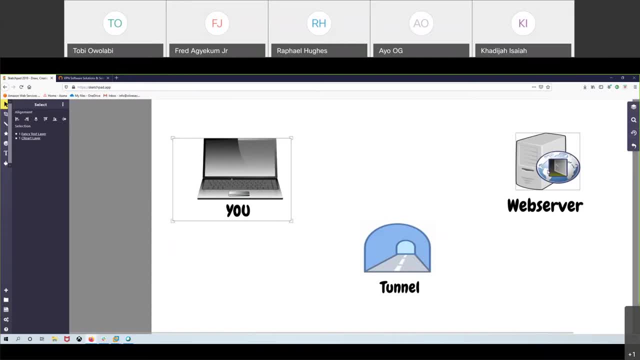 going to see it again today. If you have a VPN, what the VPN does is creates a tunnel. The VPN creates a tunnel and it encrypts all of your information, anything you're doing on the internet on that open network. it encrypts it inside of this tunnel and sends it to the web. 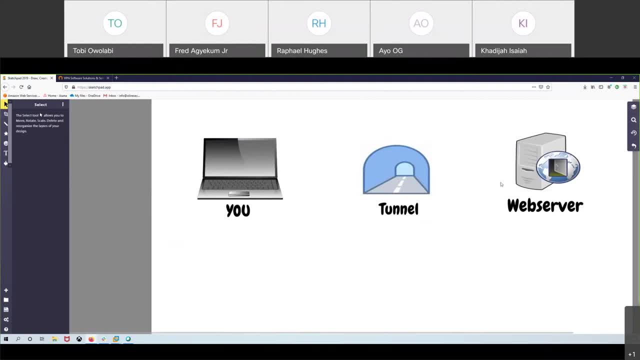 server. That's what a VPN does. Now, how it encrypts it is with IPSec. It's using IPSec to create the tunnel and encrypt the tunnel and prove that you are the person on the other end of this tunnel going to the web server, And the web server is who they say they are coming back to you. 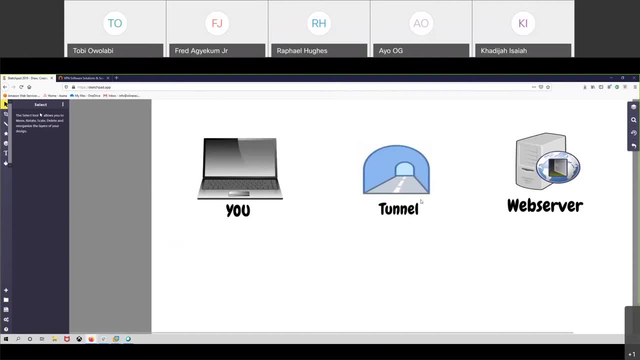 So all that IPSec is doing is giving you a secure way to communicate on open networks. It doesn't even have to be an open network. It can be an encrypted network. You just have your VPN, just because Some companies still require you to use a VPN to get into a server- web servers- 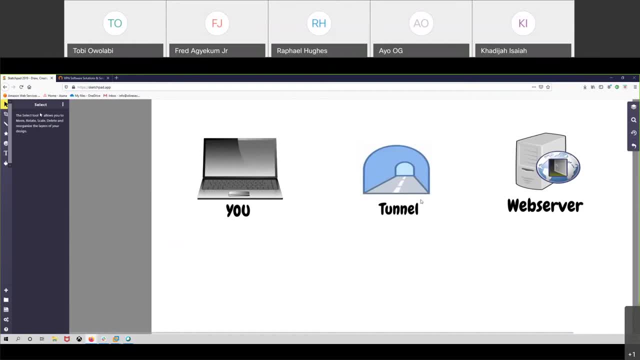 web applications, whatever, because it's just more safe on the operations side of things. So if that was clear, if IPSec was clear, if you guys don't have any other questions from the class, I'm gonna go ahead and dive into our session for today. Anybody got any questions? Yay, nay. 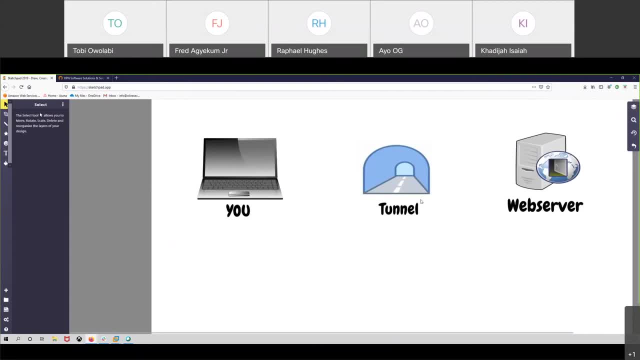 No, I understand it. Is that also? because I think he also talked about reverse path forwarding? Yeah, Is that also Okay? So I'm going to pause for a moment. so I'm going to pause because I'm going to pause for a moment. 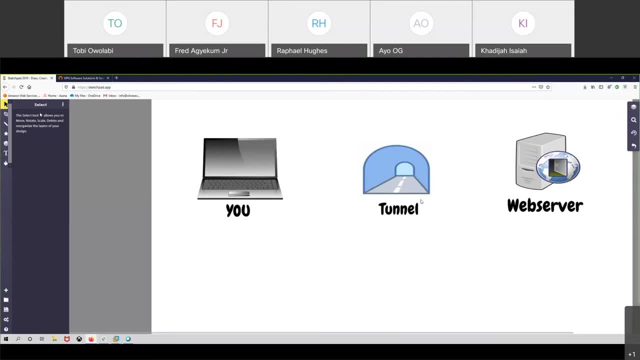 Okay, so I'm going to pause for a moment. so I'm going to pause for a moment. So I'm going to pause for a moment. so is that also when it does that, um, when it's doing a encrypting in a tunnel and it sends? 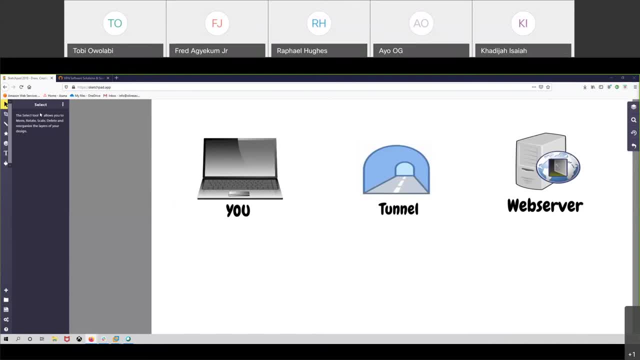 it to the web server, can it also? can it also be doing that at that time too? so reverse path forwarding is for routers, um, so that's, yeah, that's for routers, and that's just to make sure that. um, and i'm not sure if you went into. 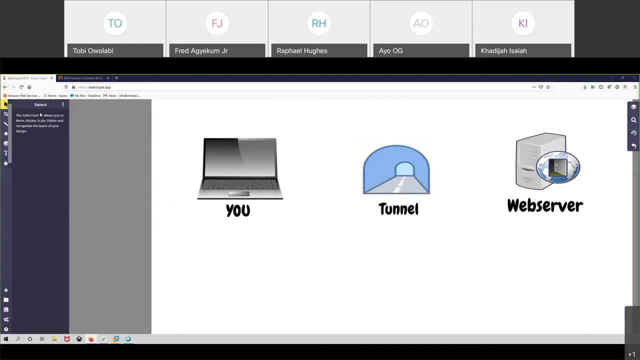 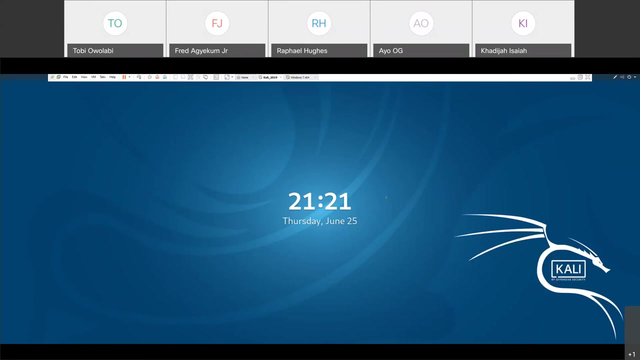 it it's, and you're not gonna need to go into too much details with rpf for the exam, especially for the exam, but it's just to make sure that your routers aren't. um. it's to prevent denial of service attacks. pretty much cool, all right. um, that's it. i'm gonna put down my picasso. 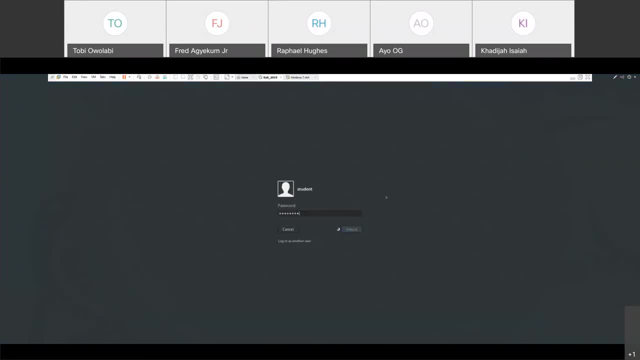 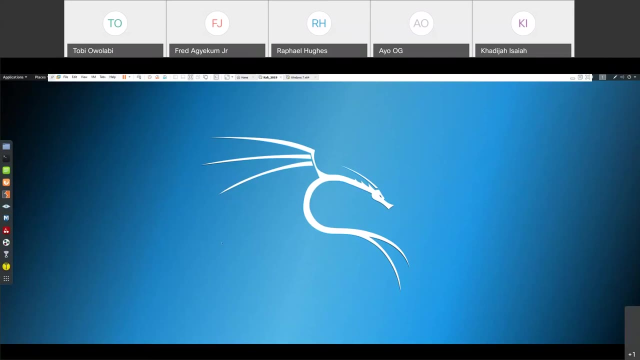 painting right there and do i remember my password? that's wrong, um all right. so what we're gonna do today, let's see i have this toolbar messing me up again on last thursday. all right, so this is. we have our cali operating system. this is our.